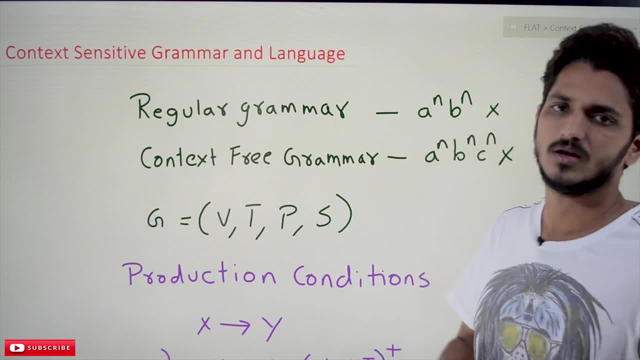 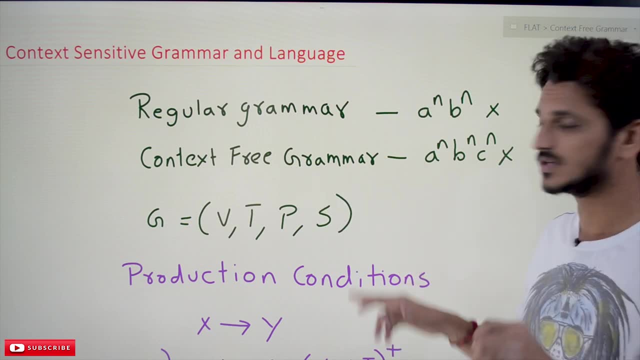 A power n, B power n. Yes, it is not defined using a regular grammar, The same way context-free grammar. We already defined about context-free grammar and we cannot define some languages using context-free grammar. One of such languages is A power n, B power n and C power n. But we can. 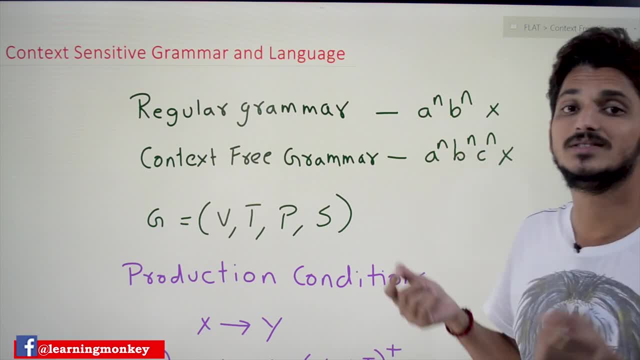 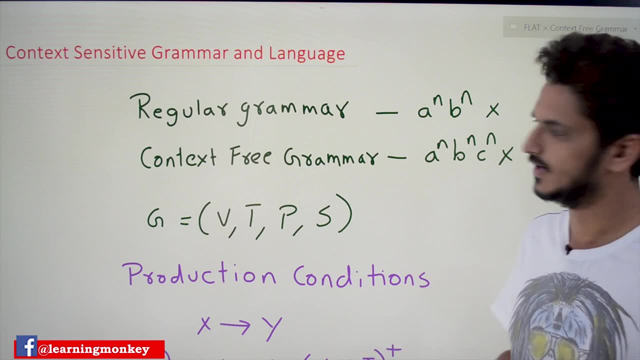 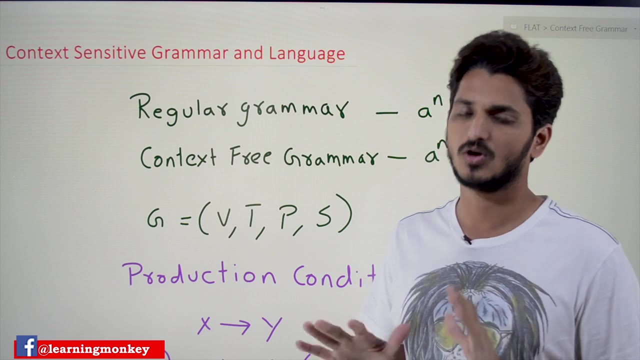 define this language using context-sensitive grammar, The languages that are able to derive using context-sensitive grammar. we call it as context-sensitive languages. Coming to the context-sensitive grammar in this class we will understand about what's the grammar conditions and a little bit about context-sensitive grammar. In our next class we will check the example. 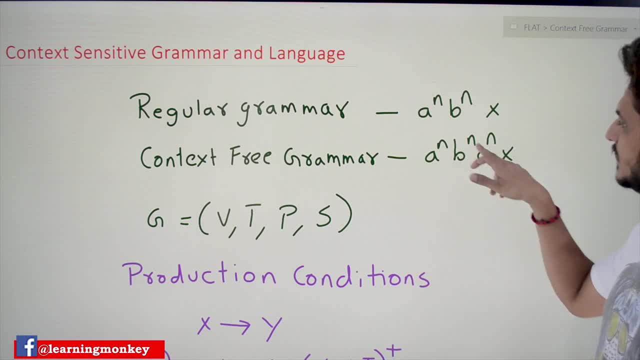 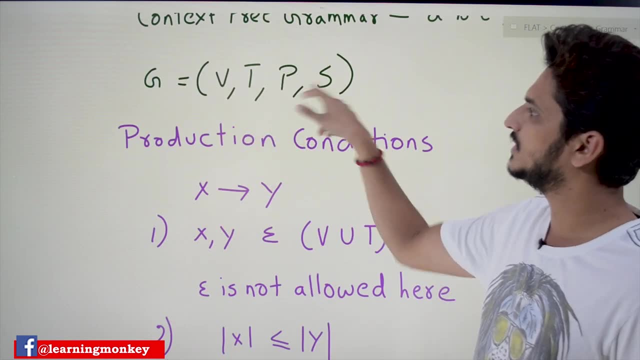 of A power n, B power n and C power n. Now let's try to understand what's context-sensitive grammar. So context-sensitive grammar consists of V, T, P, S. V means variables- We call it as non-terminals. T means 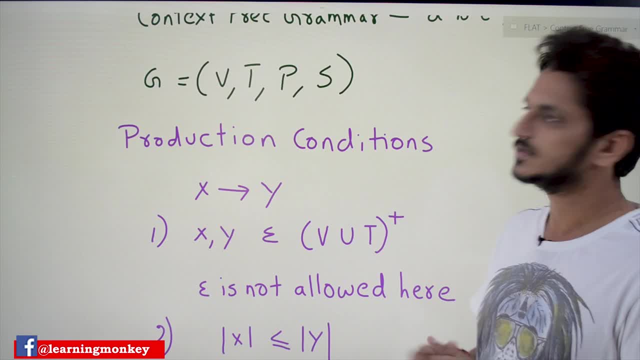 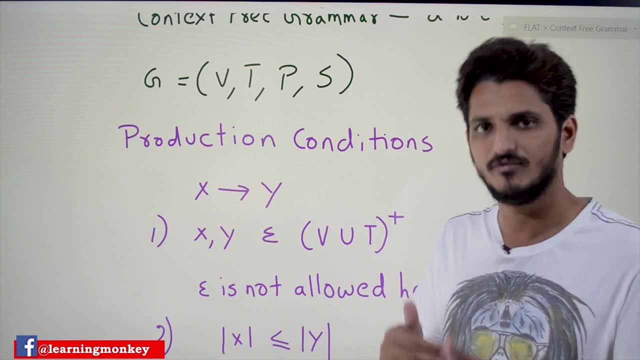 terminals. P means productions, S means a start symbol, Same way production. So what's the difference between regular grammar and context-free grammar? Production conditions: That's the difference. The same way, what's the difference between context-free grammar and context-sensitive. 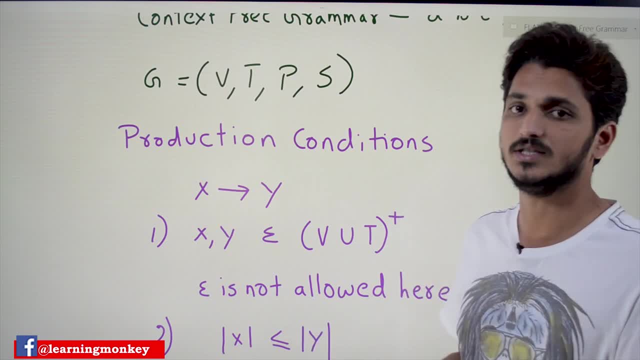 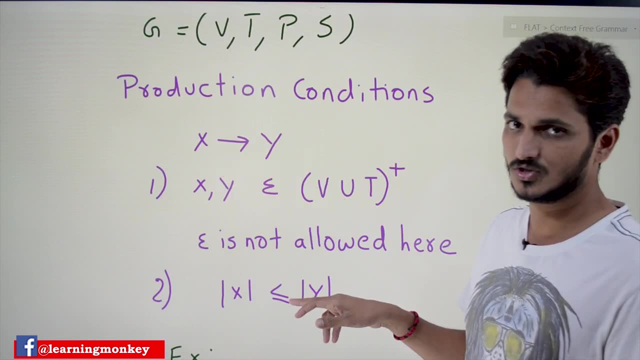 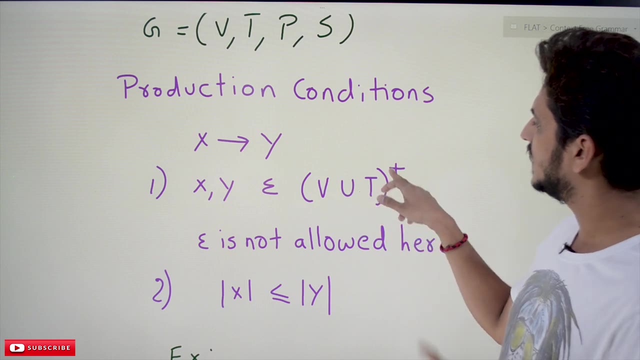 grammar. Production conditions are the difference. What's those conditions? Let's try to understand. Production conditions are: if you take X tends to Y is a production. in context-sensitive grammar it has to follow some conditions. What's those conditions? X comma, Y belongs to V, union, T, whole. 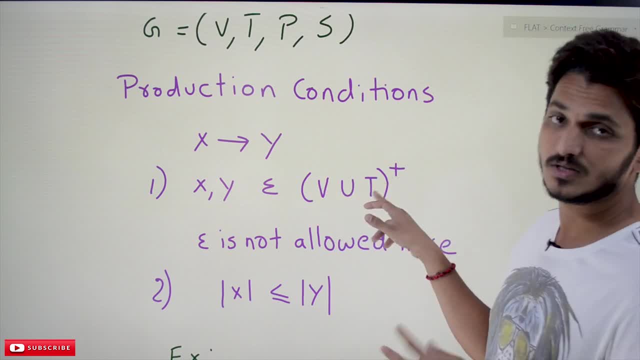 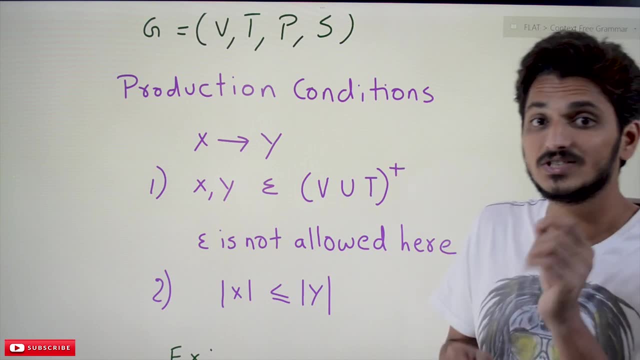 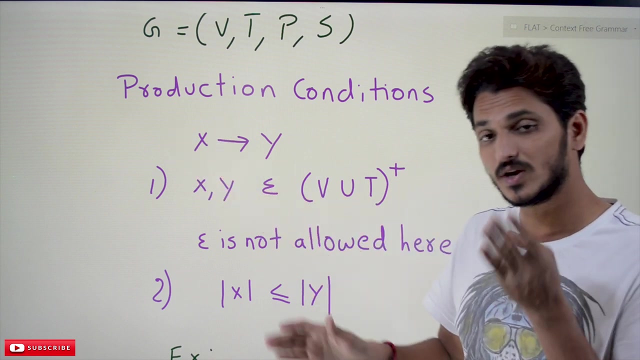 plus V means non-terminals, T means terminals Means combination of terminals and non-terminals. You can take any terminal or non-terminal. Whole plus means at least one symbol should be there. That is what this condition says Means on the left-hand side. you should have at least one. 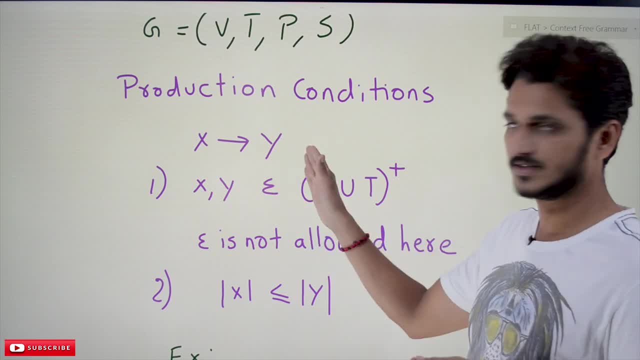 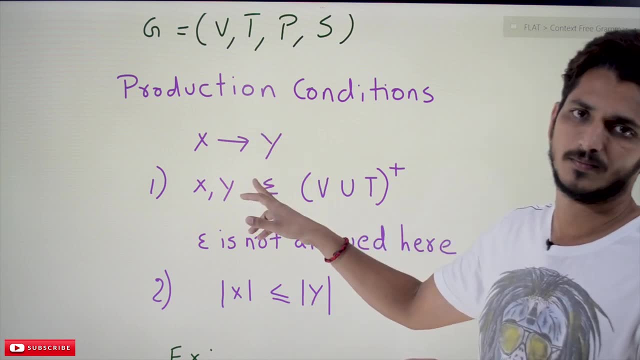 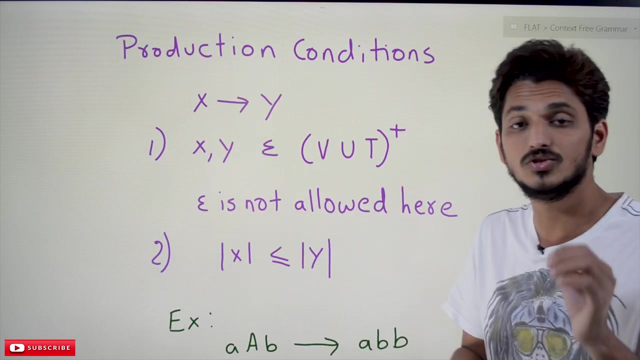 terminal or non-terminal. On the right-hand side you should have at least one terminal or non-terminal. That is what context-sensitive grammar condition is One of the condition. From this condition we can understand that epsilon is not allowed here- Context-sensitive. 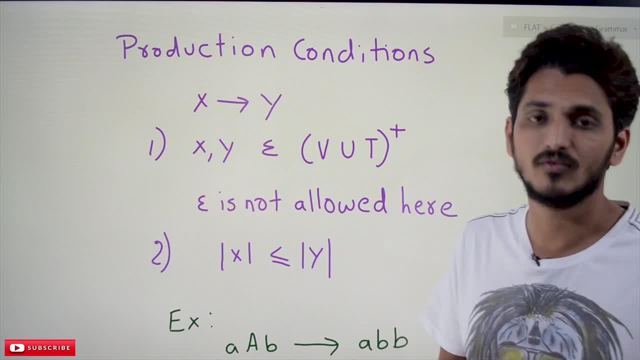 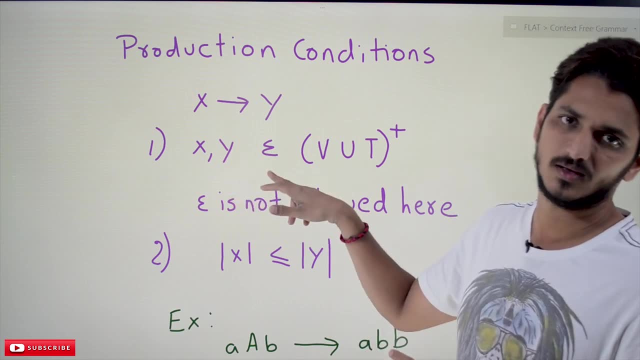 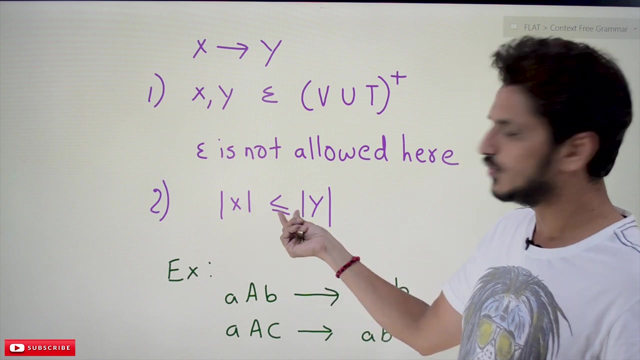 grammar. it won't allow epsilon in the language, Means in the language it won't accept epsilon. That is what this condition says. The second condition is the length of the left-hand side production should be always less than or equal to the length of the left-hand side production. 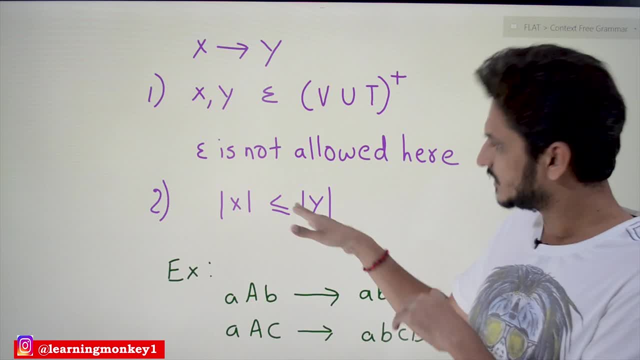 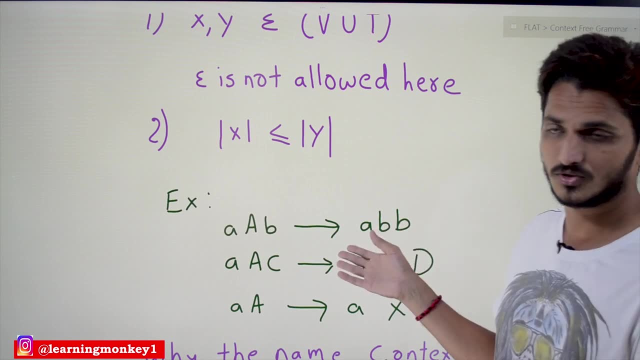 equal to the length of the right-hand side production. Try to understand this with an example: AAB tends to ABB. Yes, this is a context-sensitive grammar. You can have anything on the left-hand side, You can have anything on the right-hand side, But the length, how many? 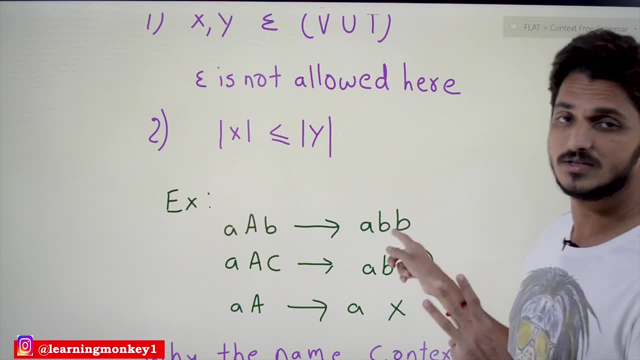 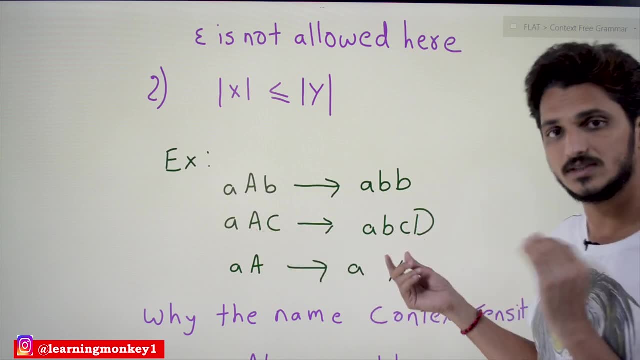 symbols. are there? Three symbols are there. How many symbols are there? Three symbols, Yes, it is accepted. On the left-hand side: how many symbols? Three symbols. How many symbols? Four symbols, Yes, it is accepted. X should be always less. 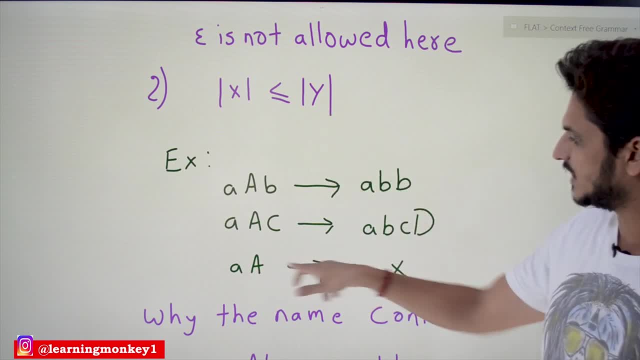 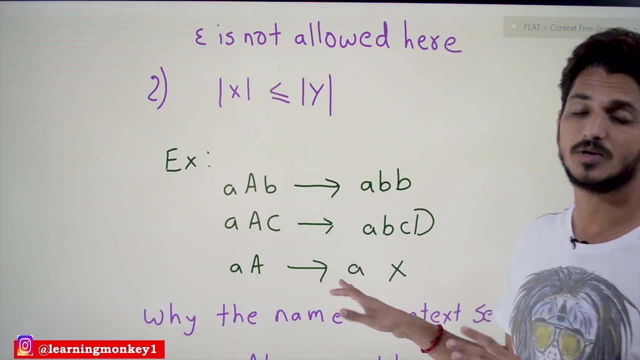 Then are equal to Y. But this is not a context-sensitive grammar. AA tends to A Left-hand side. we are having two symbols. On the right-hand side we are having single symbol. It is not accepted. Always the length on the left-hand side should be less than or equal to the length. 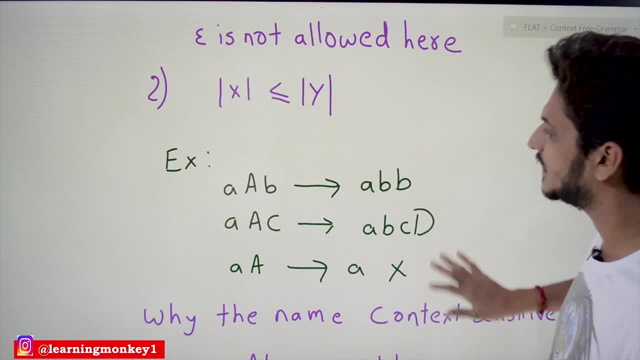 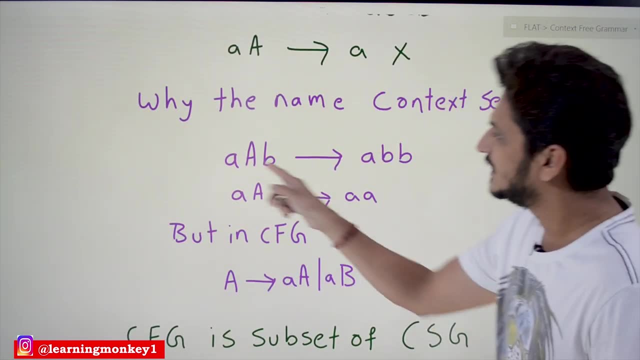 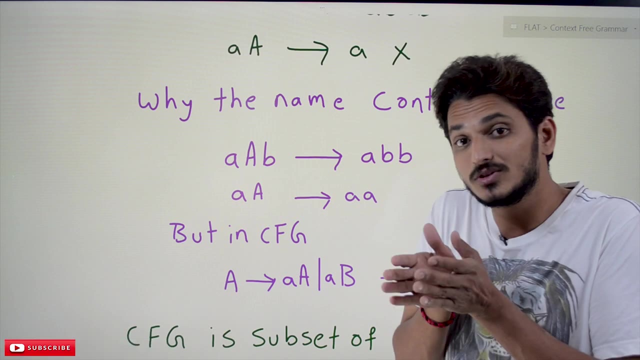 of the right-hand side. These two conditions should be followed by the context-sensitive grammar. So why we got the name context-sensitive? See here: A non-terminal A followed by terminal A. We are applying A based on some context. So what's there on the left-hand side? What's there? 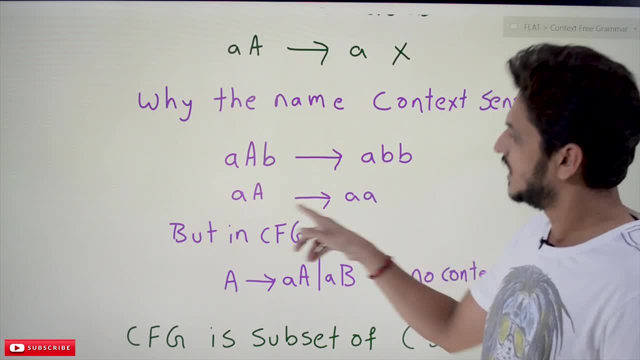 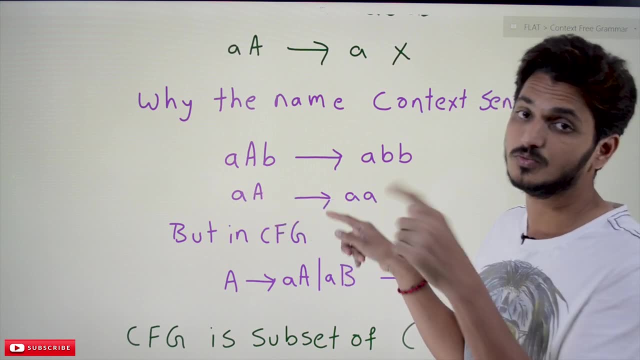 on the right-hand side. Based on that, we are applying the production If A on the left-hand side. if you are having A, we are applying this. That's why it's got the name context-sensitive. But when but you take the example of context-free grammar: whenever you see A, you can apply this. 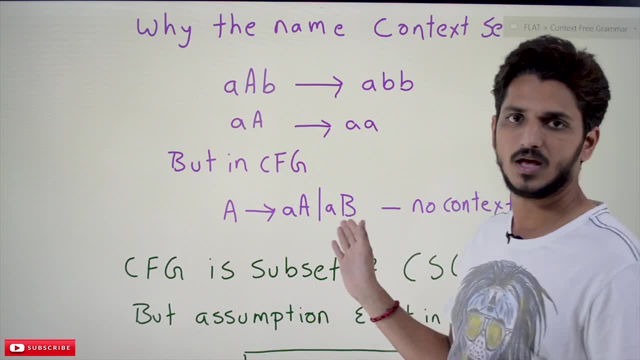 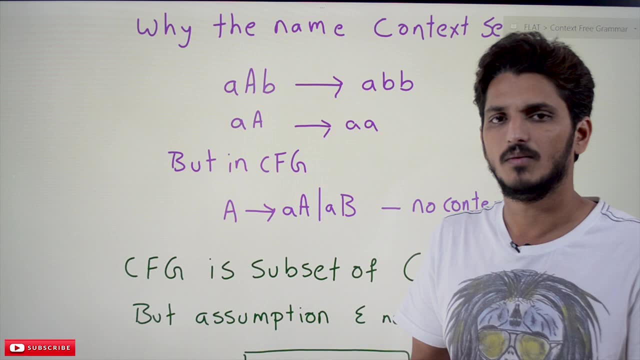 or that, Based on the situation, we go with this or that. We are not taking any context. What's before A, What's after A? That context is not considered Blindly. we will see A and we will apply either this or that. We will check the context If this is not satisfied. 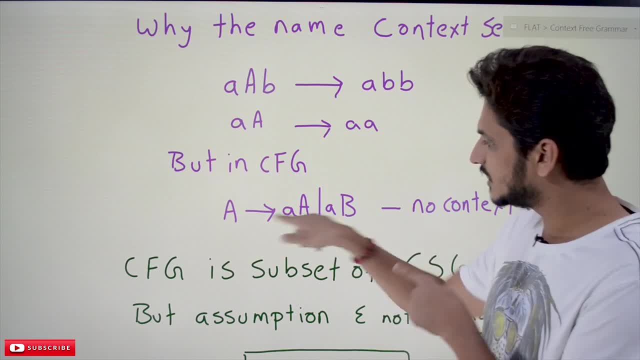 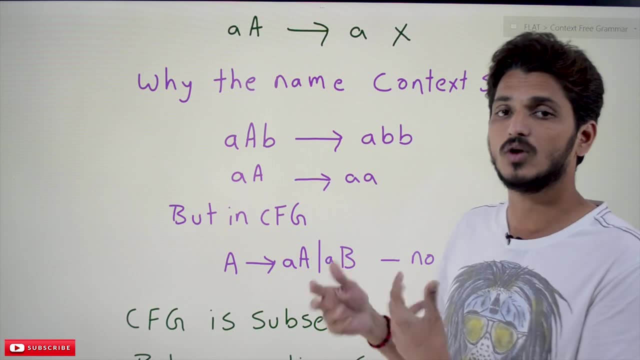 this. we go with this. So that's why it got the name context-free grammar, Why we call it as a: Because it is checking the context also On which context we are going to apply A. That's why it's got the name context-sensitive grammar. 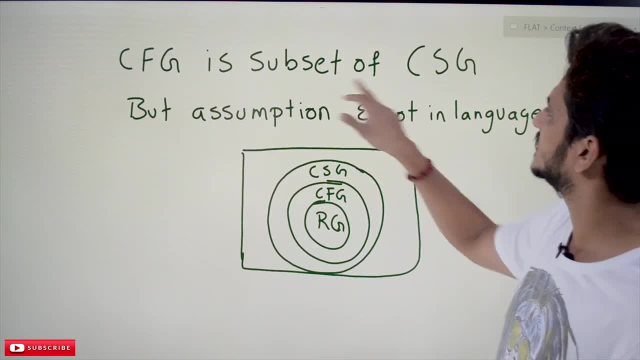 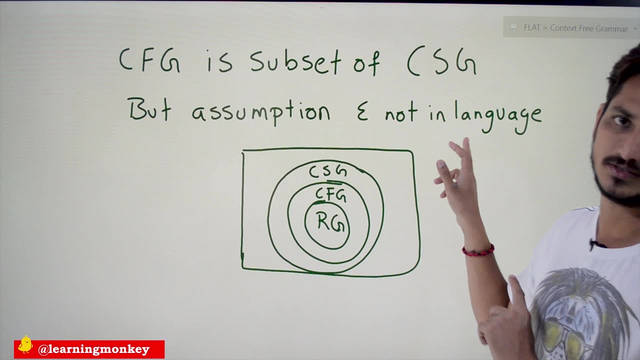 Now, coming to the next point you have to understand. context-free grammar is a subset of context-sensitive grammar, But there is an assumption that epsilon is not in the language, Then only this condition satisfies. So context-free grammar is subset of context-sensitive.